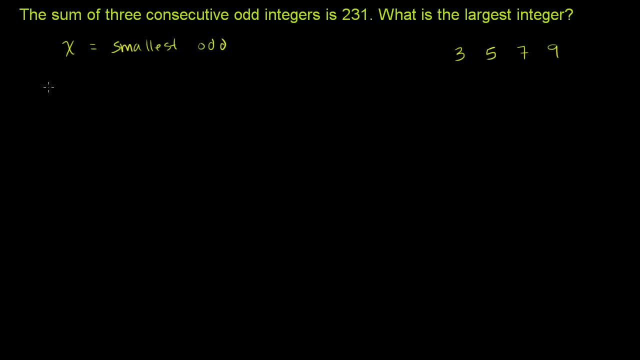 So every time we add 2.. So if the smallest one is x, the next smallest odd integer is x plus 2 is equal to the next smallest odd integer. I'll write integer here, Odd integer, And then what will be the next one? 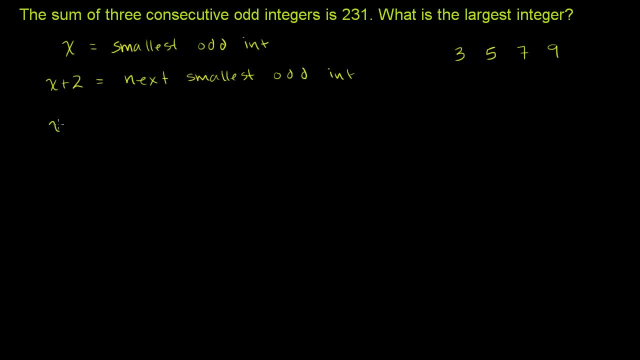 Well, we're going to add 2 to this one, right? So it's going to be x plus 4.. Think about it: If the smallest is 3,, then we have x plus 2,, which is 5.. And then you have x plus 4,, which is 7.. 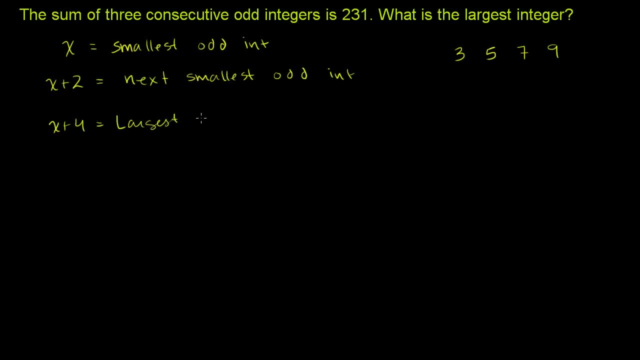 So this will be the largest of the consecutive odd integer in this group, And they tell us that the sum of these consecutive odd integers is 231.. What is the largest integer? So if I take x, x plus 2, and x plus 4, and I sum them, they 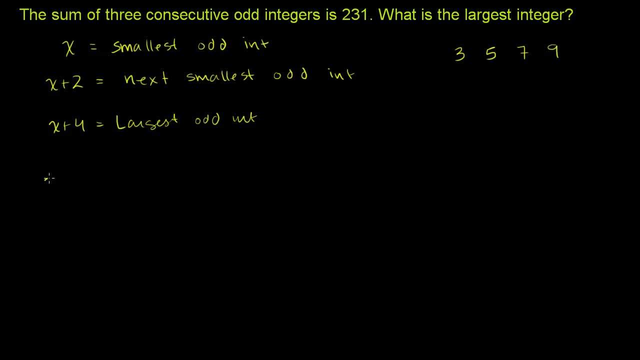 should be equal to 231.. So let's do that. So we have x plus x plus 2 plus x plus 4.. And this needs to be equal to 231.. And when they ask us what's the largest one, we're going to. 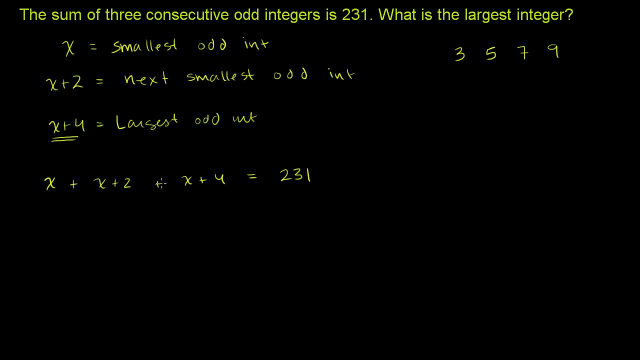 have to tell them what x plus 4 is equal to. So let's just solve this equation. So let's add our x terms. We have 1x, 2x, 3x's, So we get 3x plus. and then what are our constants? 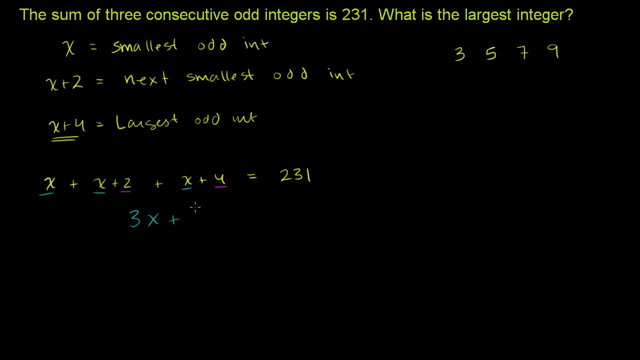 We have a 2 and we have a 4.. So 3x plus 6 is equal to 231.. Now let's get rid of the 6 from the left-hand side of the equation. Best way to do that is subtract 6 from both sides. 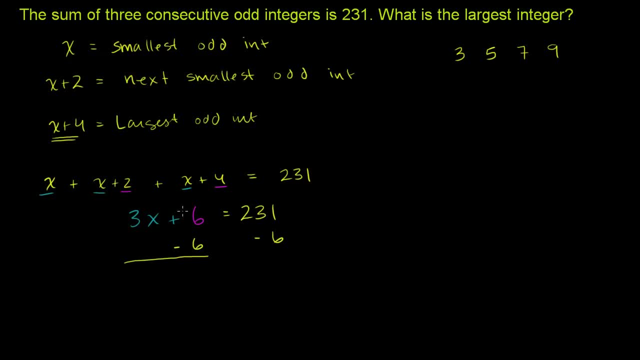 So let's subtract 6 from both sides- The left-hand side- we're just left with a 3x. The 6's cancel out The right-hand side: 231 minus 6 is 225.. We get 3x is equal to 225.. 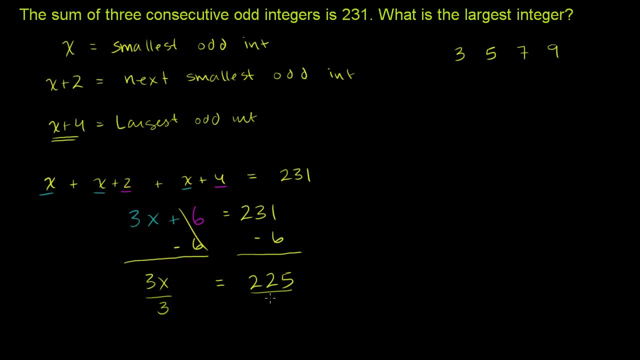 To isolate the x, let's just divide both sides by 3.. The left-hand side, the 3's, cancel out. That was the whole point behind dividing by 3.. We get just an x is being equal to and 225 divided by 3..